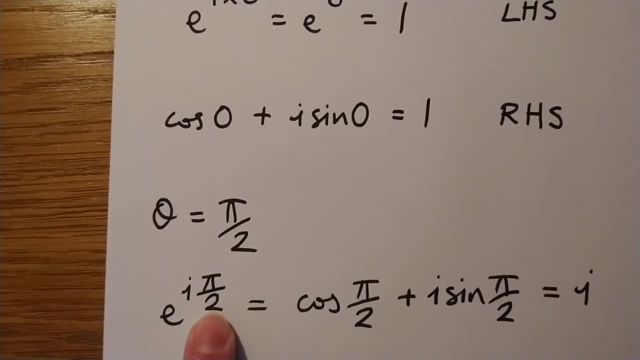 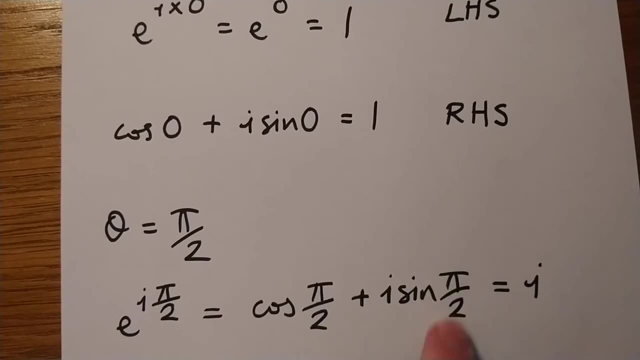 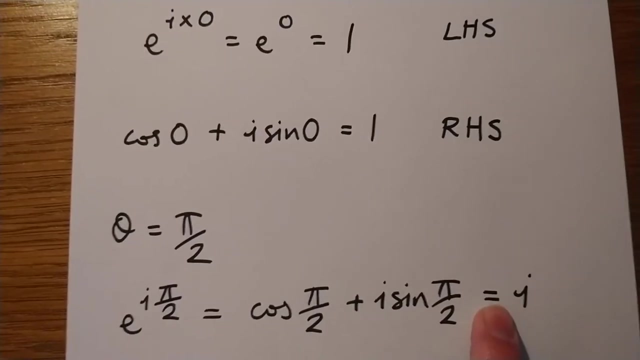 to kind of expand this, which we're not going to do in this video. But let's look at the right hand side. That would give us cos of pi over two plus i sine pi over two. So that's the right hand side. Well, cos of pi over two is zero, Sine of pi over two is one. so we get the value i Now, if we make, 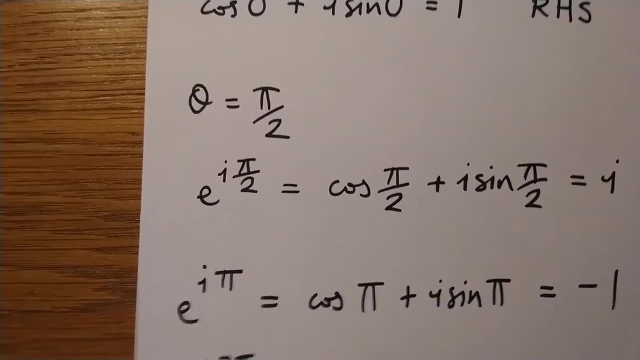 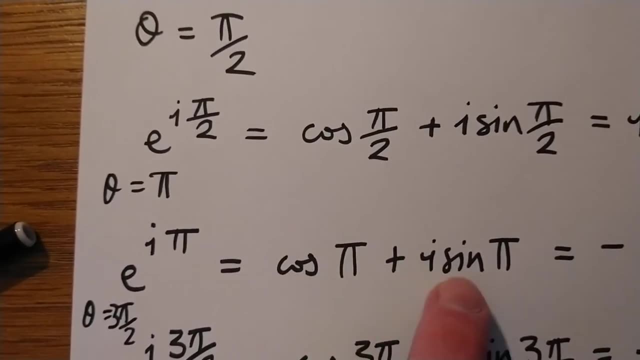 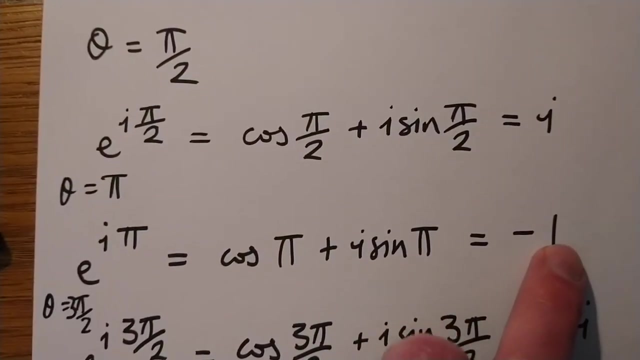 theta equal to pi. I'll put that in there. actually we have e to the. i pi is equal to cos pi plus i sine pi. Well, sine pi is zero. so the imaginary part disappears. Cos of pi is negative one. Now one more. 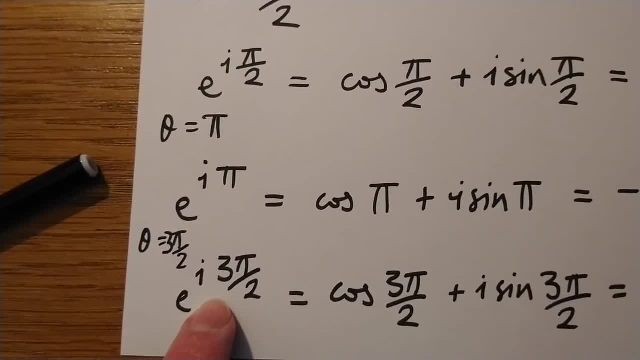 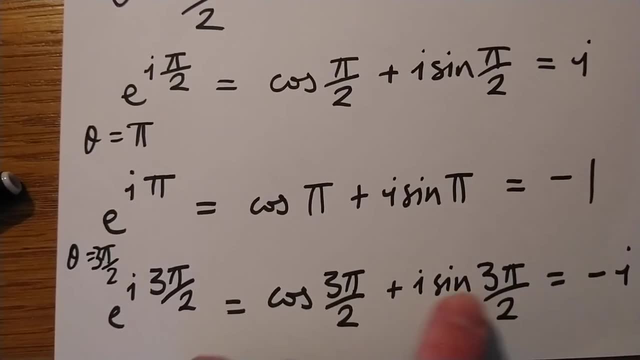 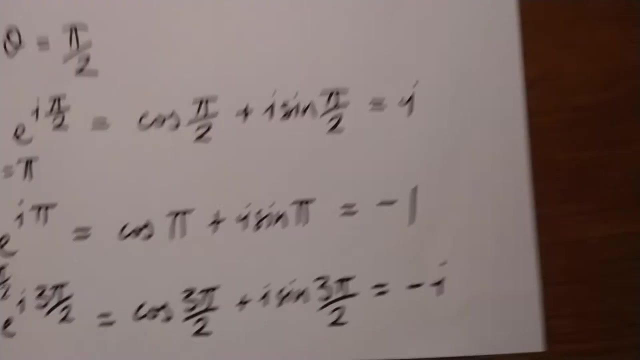 If theta is equal to three pi over two, then we have e to the i. three pi over two is cos of three pi over two, plus i sine three pi over two. This one is zero, but this one is equal to negative one, so we end up with negative i. So let's take a look at those four. on the Argand diagram. 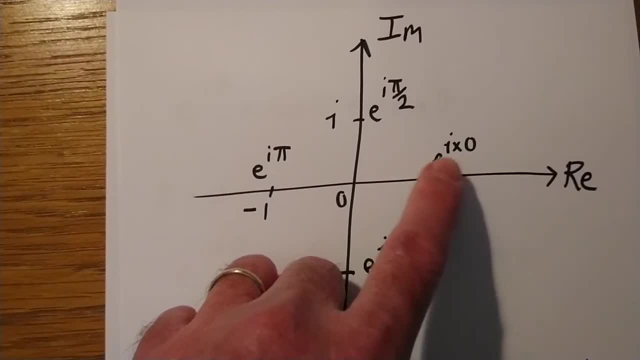 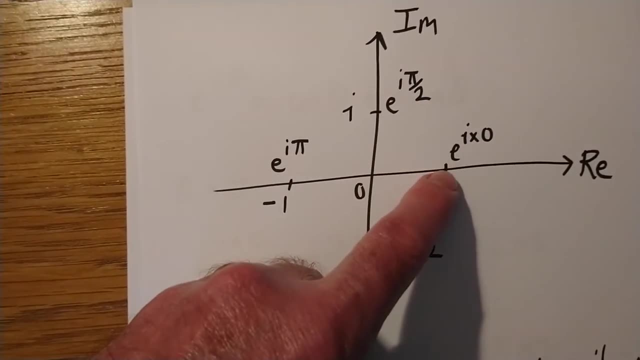 So we've got e to the i pi, sorry, e to the i. multiplied by zero here that's equal to one. If we go to e to the i pi over two. notice the argument of that would be pi over two and the value is i. 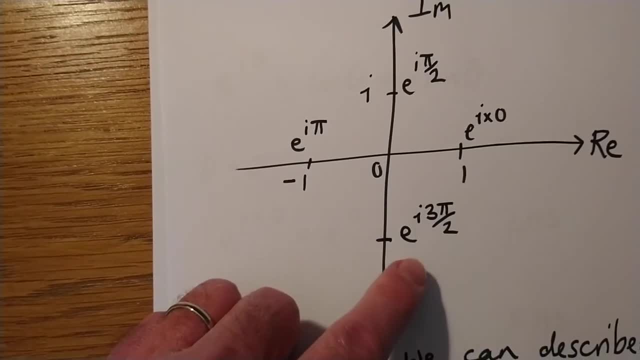 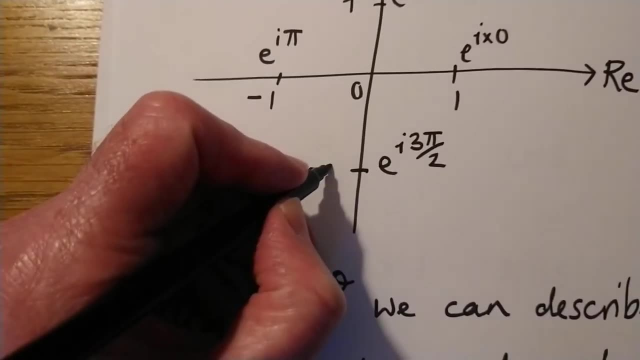 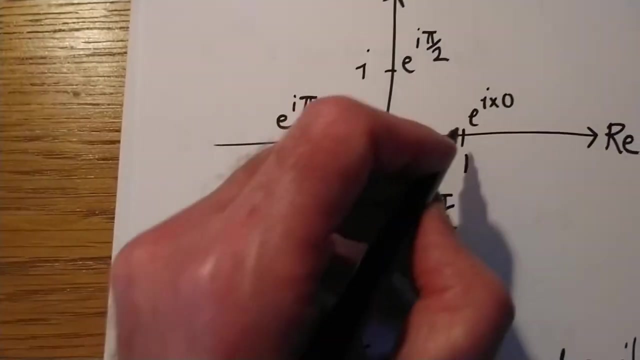 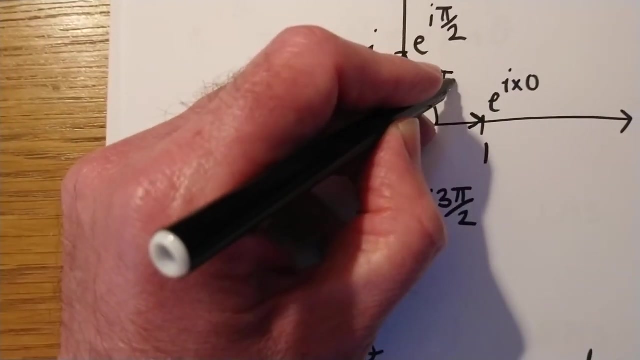 e to the i pi is negative one and e to the i three pi over two is minus i. Okay, so notice that the angle we put in here, if we were to draw a little vector, it's always the angle that is the argument of the complex number. 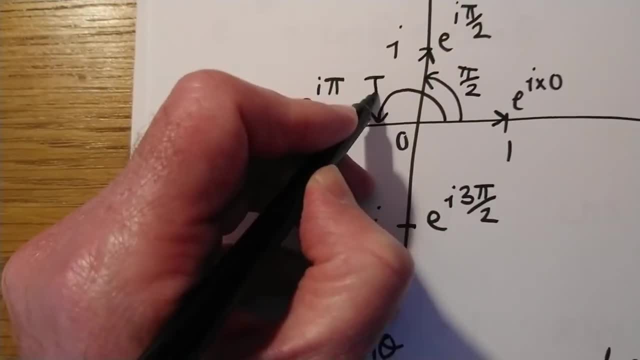 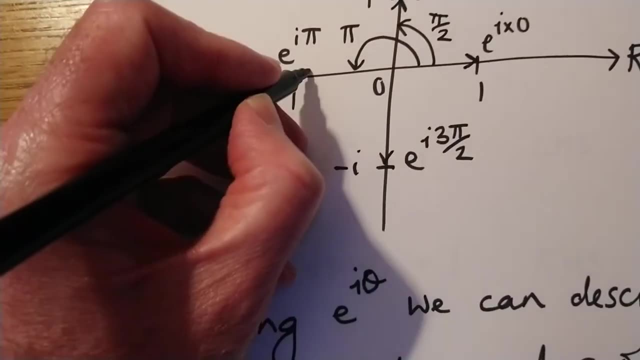 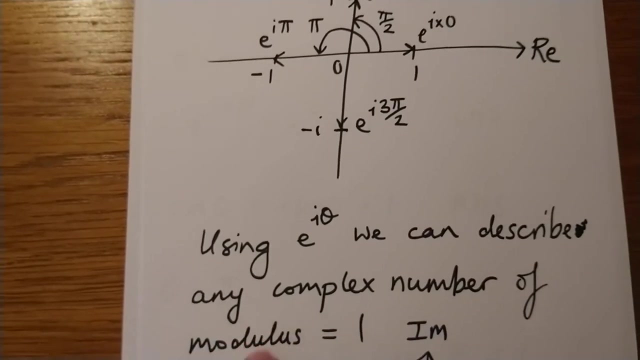 Okay, so for e to the i pi, we've got pi radians going around there and we'd have three pi over two if I drew in the vector that's pointing straight down here. So using e to the i theta we can describe any complex number, providing the modulus is equal to one. 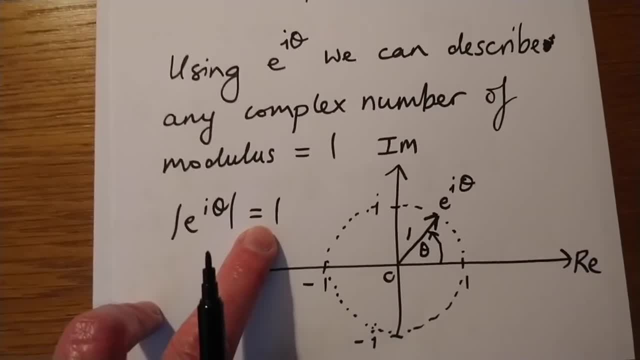 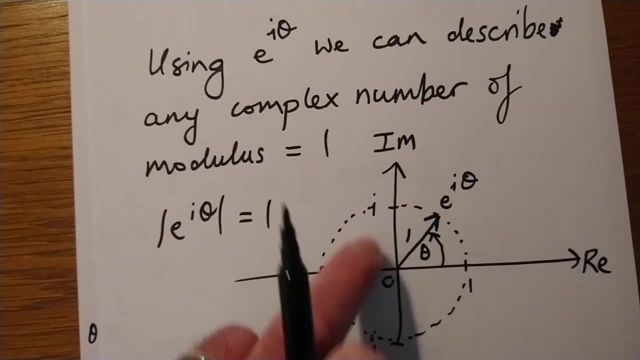 So the mod of e to the i theta is always going to be equal to one and we kind of map, we could kind of map out a circle with that little vector, that complex number. So if we plot e to the i theta, we know the modulus is going to be: 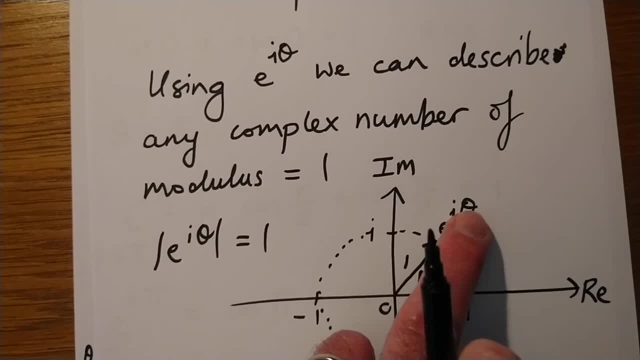 one and whatever angle we put in here in radians, that's going to be the argument of that same complex number.